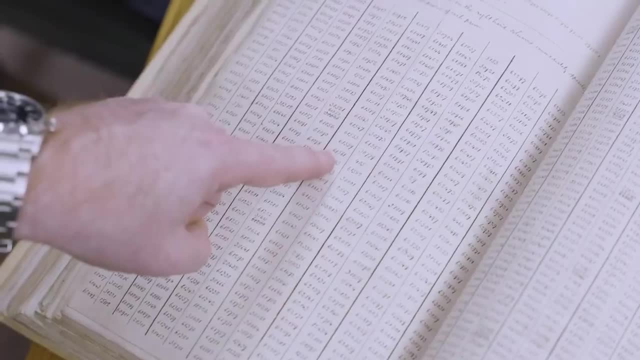 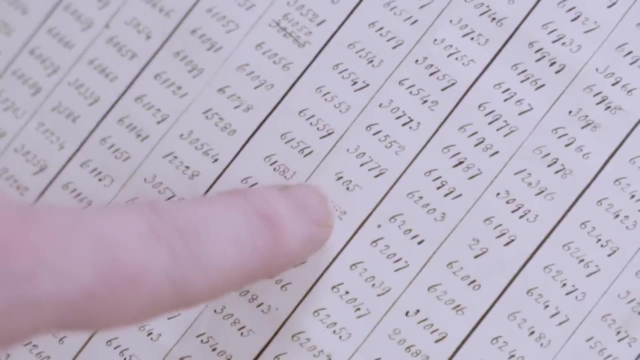 So give me a prime and I'll put it in here and see what it says. I'm going to pick 61,561.. That has 405 digits. What have we got? 405.. Correct, Shanks and Shanks bot agree. So I tell you we'll do one by hand. 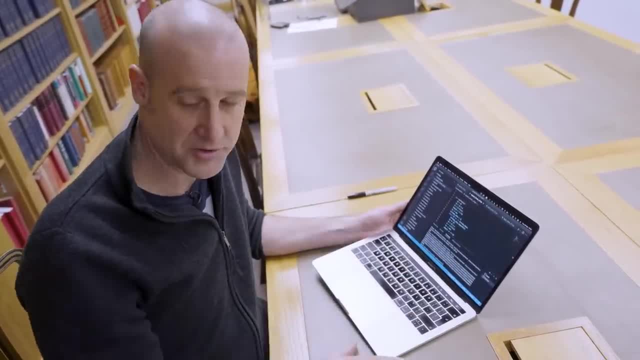 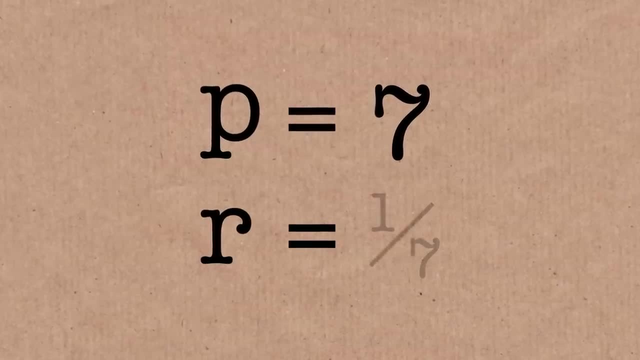 and I'll show you what the Shanks bot is doing, and that'll show us what the worst-case scenario can be. Okay, So we'll start with The prime 7, which means the reciprocal of that prime is 1 over 7.. 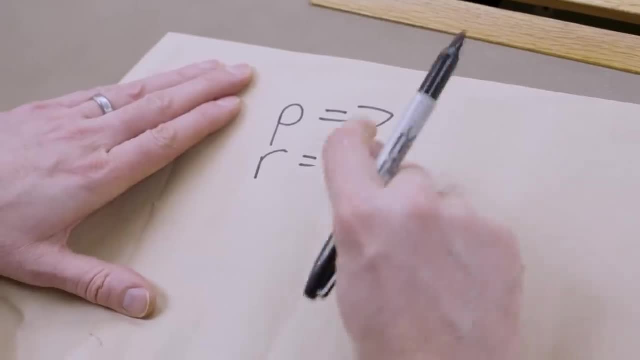 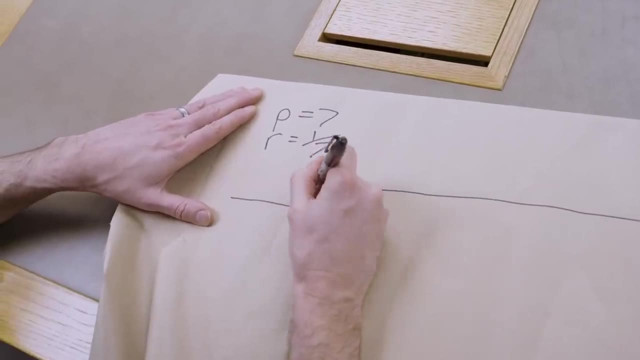 And this means 1 divided by 7, or in primary school terms, how many times does 7 go into 1?? So let's do it as a long division. So here you've got your divot end. That's the number going into it, And here you've got the number you're dividing it into. 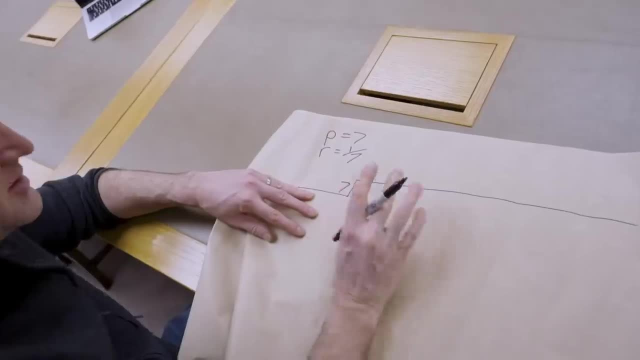 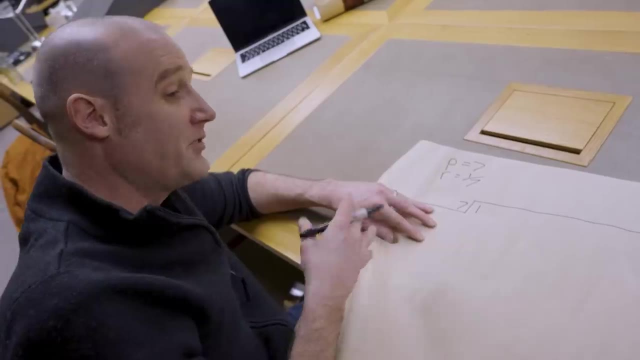 So it's 7 into 1.. Now the issue is: 7 does not go into 1, because this is not very groundbreaking. 7 is bigger than 1. We have a problem. However, We can try and work out what fraction of it is going to go in. 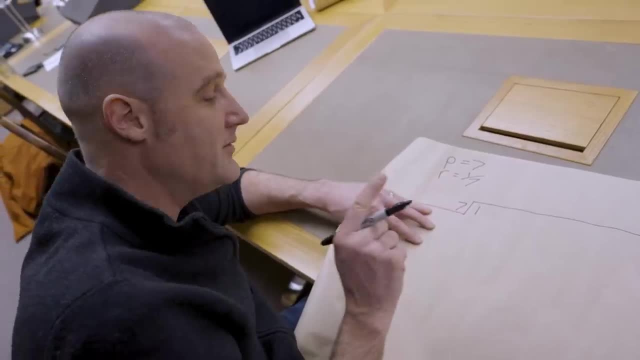 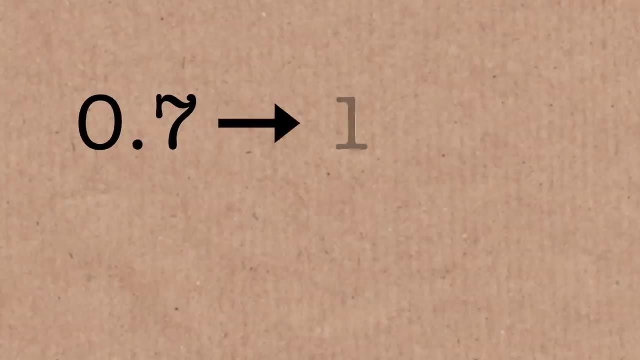 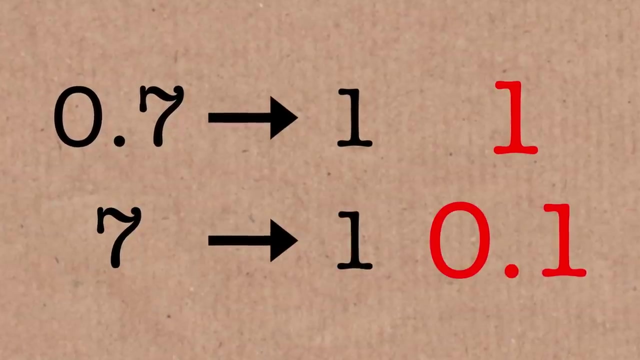 And so, actually, while 7 doesn't go into 1, 0.7 does go into 1.. So if I say 0.7 goes into 1 once, that's the same as saying 7 goes into 1- 0.once. 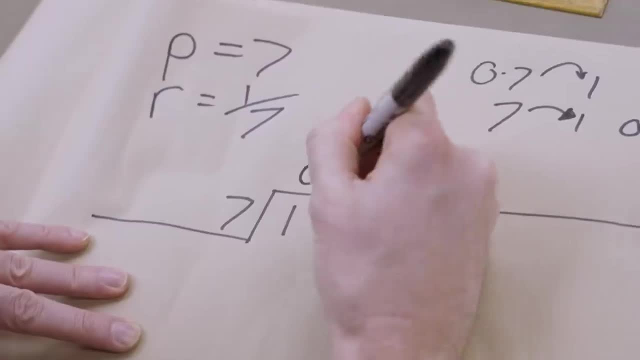 So what we're saying is: 7 goes into 1, 0.once, but it's got a leftover- 0.3.. So what we do now is we're going to put our, We're going to put our leftover down here. 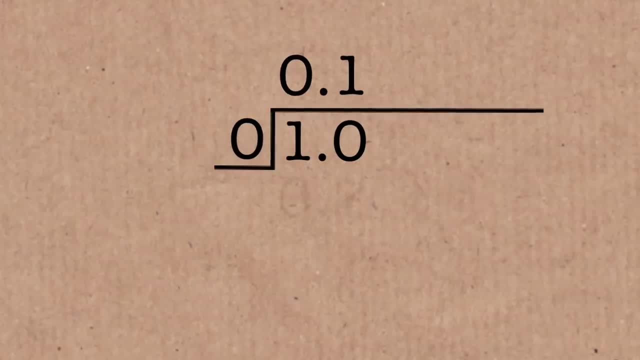 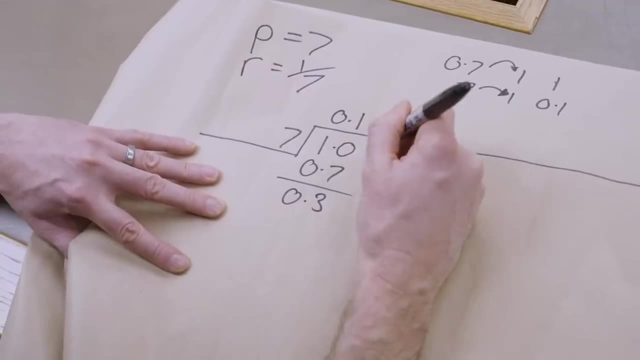 What we've done is we've said: if you've got 1.0 and you put in 0.7, what you're left with is 0.3. And now we're going to repeat that Implied are all these extra zeros right. 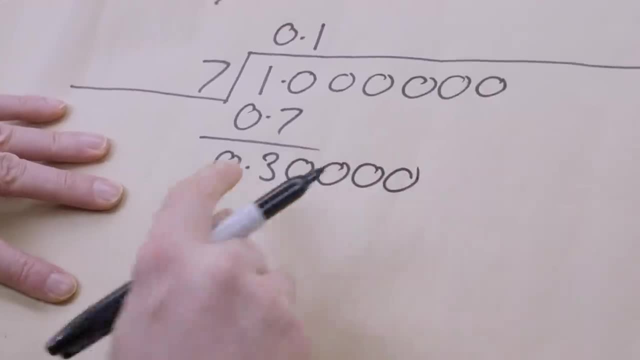 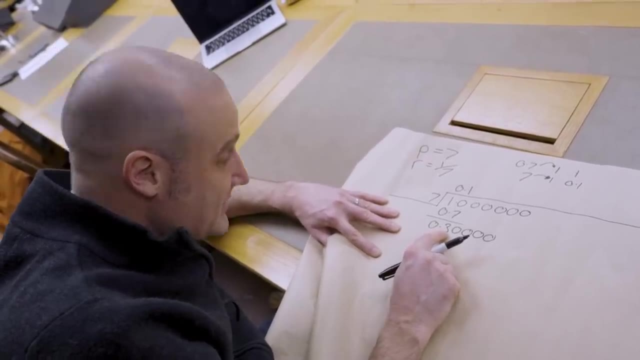 Because there's infinitely many of these, which is very convenient. We just need to know- now we've already covered this bit- how many times 7 goes into that. And now we're like, okay, we can't do. 7 doesn't go into 0.3.. 0.7 doesn't go into 0.3, but 0.07 does. 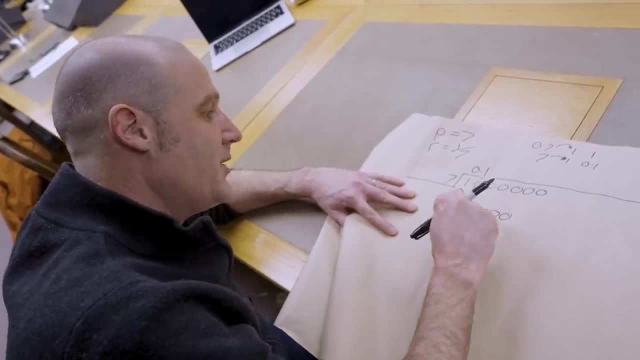 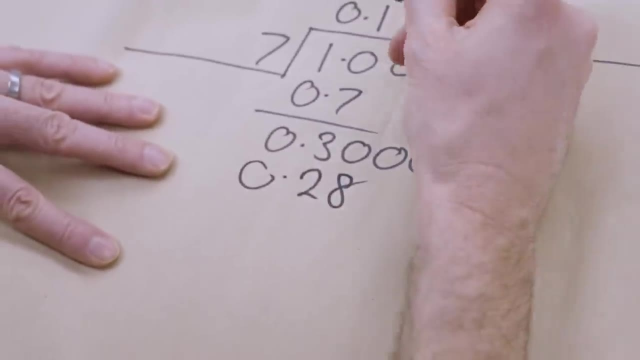 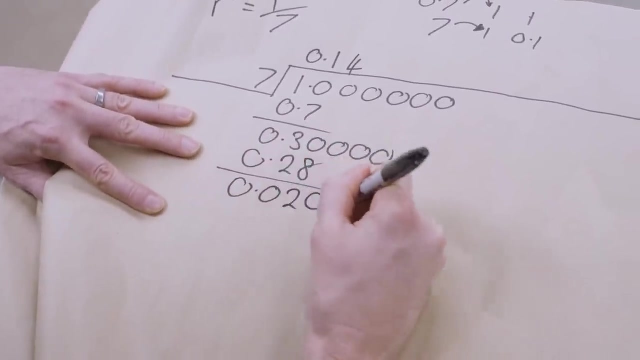 And so you go. how many times does 0.07 go in? Well, 4 times 0.07 is 0.28, and that's 4 times it. so we put it up here and then we subtract that off and we've got 0.020.. 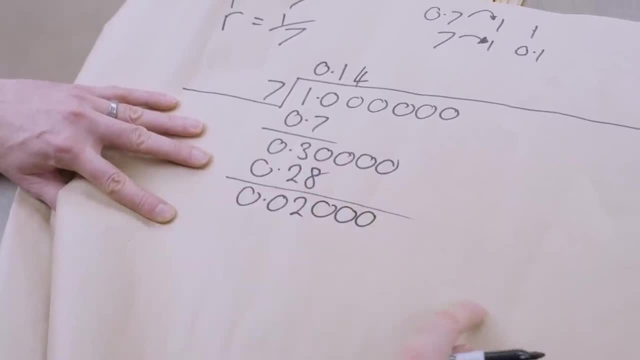 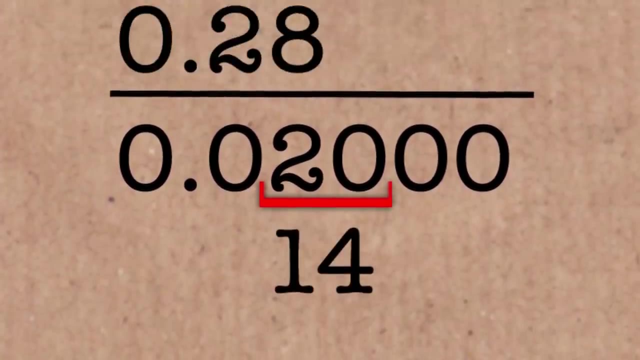 Now, at this point, we actually don't need to write in all these zeros every single time. All we really care about is the 2 and the 0 after it there, all right, And so we go. how many times does 7 go into 20?? 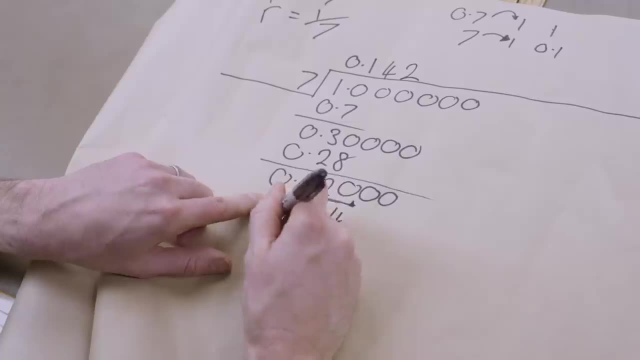 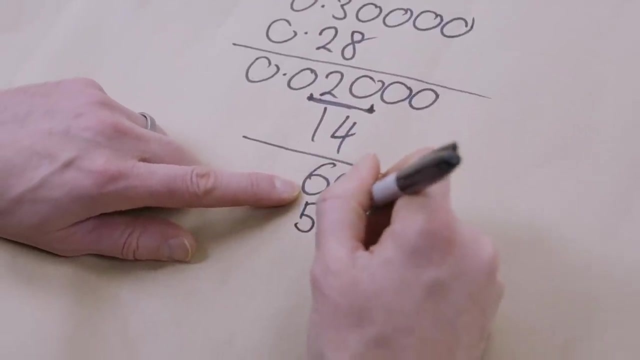 Well, it goes in twice, it's 14.. Put the 2 up there, subtract that off, We've got 6.. Now we can add on one of these extra spare zeros, of which there are infinitely many. 7 goes into 50, that's 8 times. 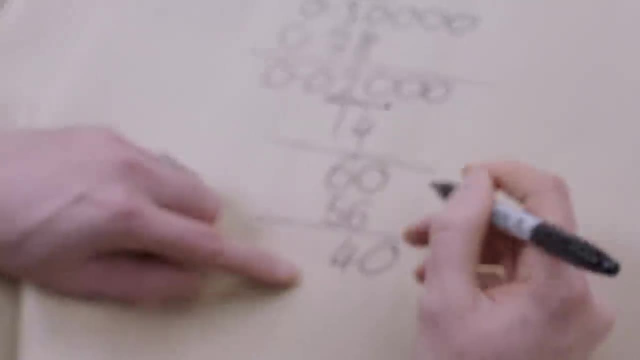 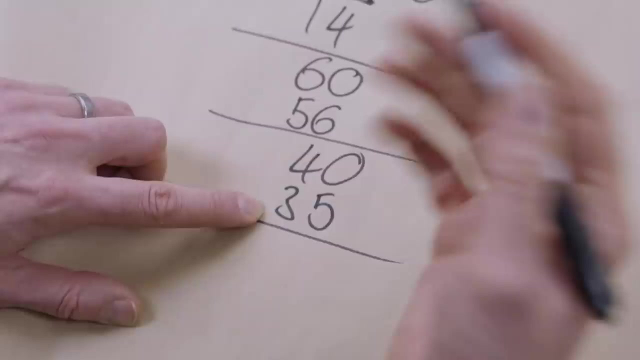 Put the 8 up there, subtract that off, It's 4.. Now it's 40.. 7 goes into 35,, 5 times. Put the 5 up there And all I'm doing is the same logic as before, but now it's just a bit more algorithmic, it's a bit more straightforward. 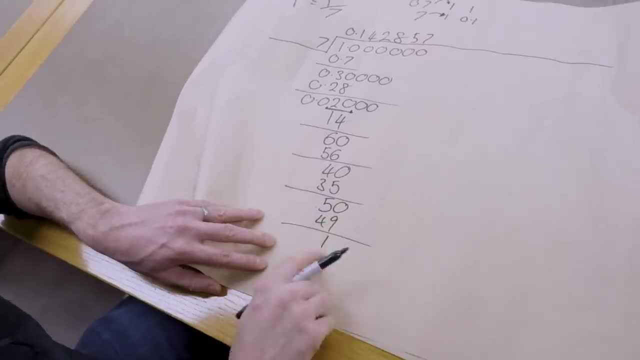 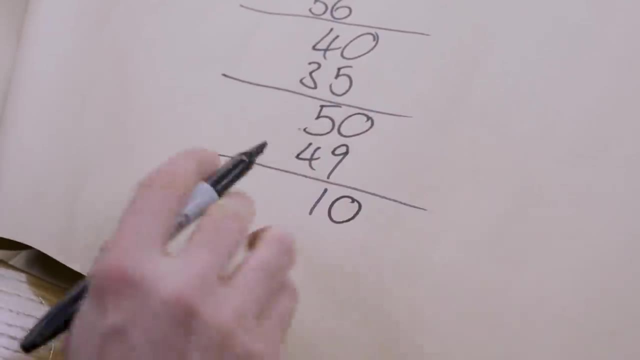 49,, 7, 1.. Ah, That's familiar. That's what we had before. So now, actually, we've got exactly the same situation down here. We're now with 7 going into 10.. Before I was faffing around with the .7s: 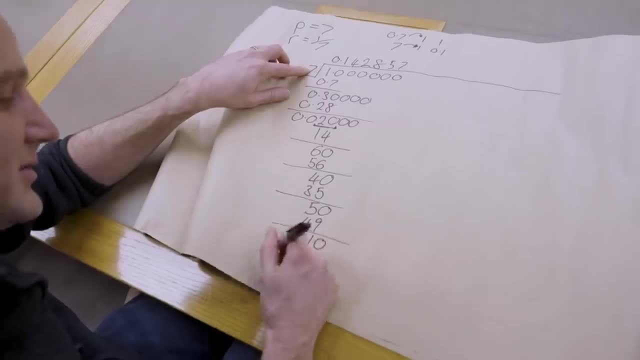 Basically, what we're going to say is: 7 goes into 10 once That's 7.. It's got a remainder of 3.. The 1 would go up there. As you can see, we've now got exactly the same here. 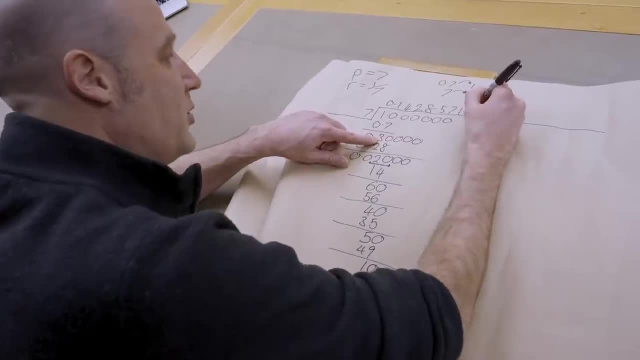 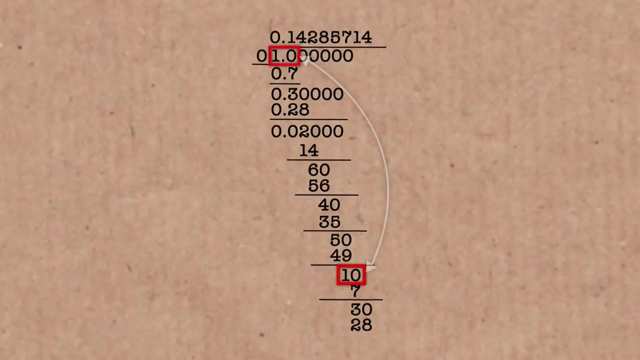 30 would have 28 underneath. We'll put another 4 there, And as soon as we hit here, that is exactly the same as what we started with here: 1 and a 0.. And so this takes us back there. 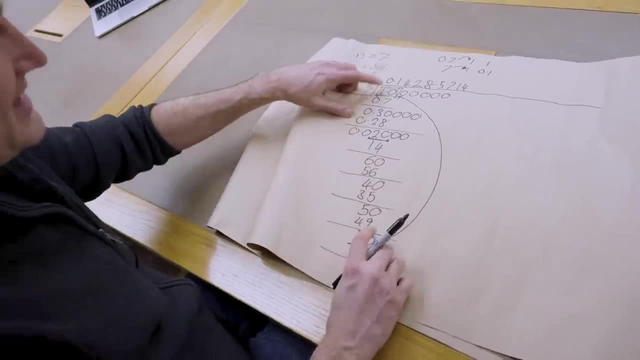 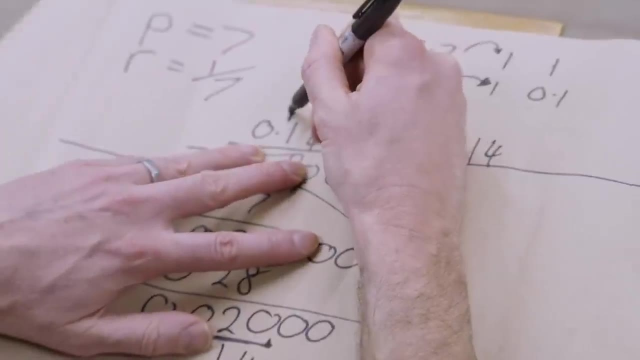 In theory it's carrying on down here, But because we've got exactly the same situation, all these steps will follow in the same order every single time, which is why 7 repeats after 1,, 4,, 2,, 8,, 5, 7.. 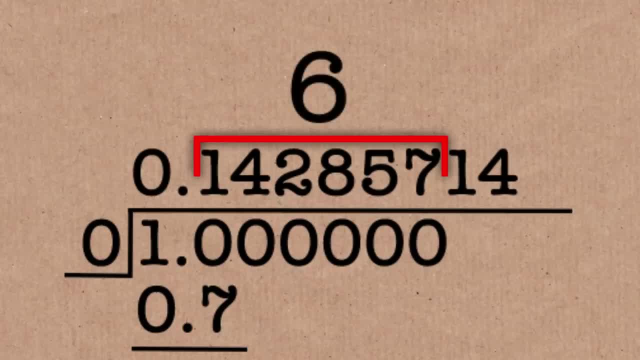 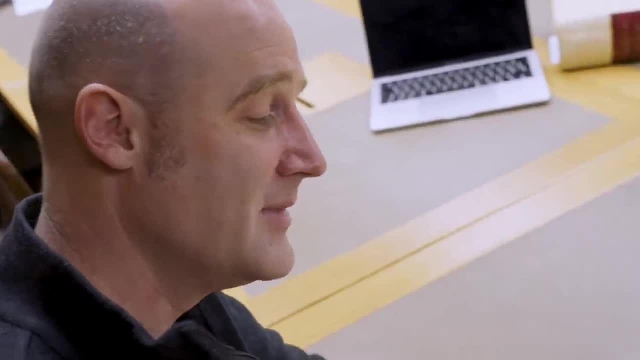 And that's 6 digits. That's when it hits this infinite loop. Will all primes hit an infinite loop like this, though? Yes, And let's do a slightly bigger one, And we'll be able to see why it has to happen eventually. 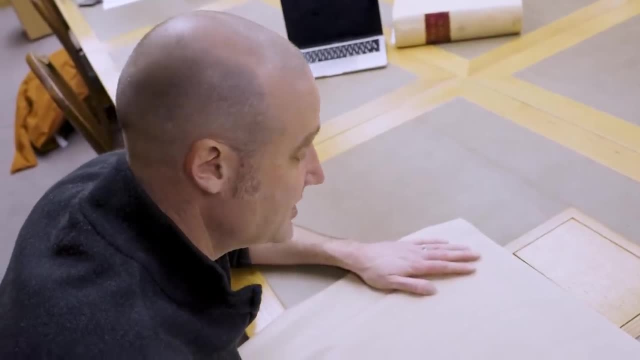 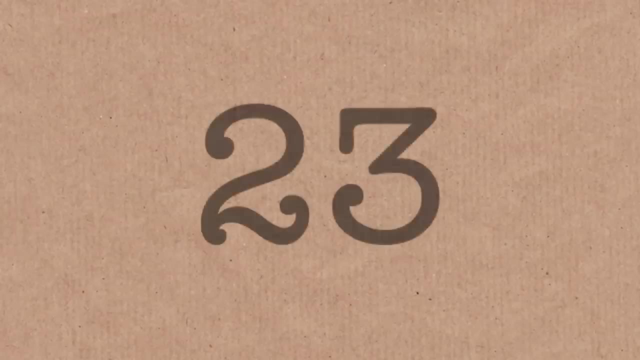 So, Brady, here's what we're going to do. We're going to try and find the reciprocal of a bigger prime. Let's keep it to 2 digits. What would you like Um 23?? 23!, That is a prime. 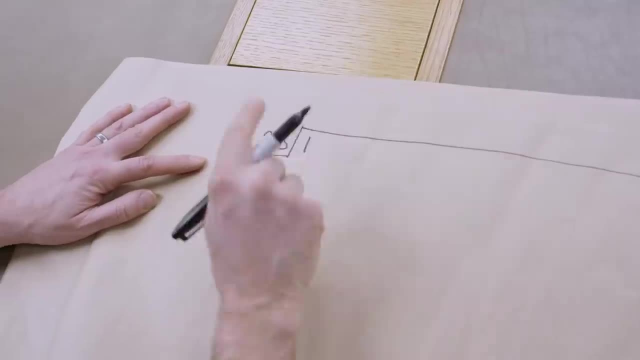 We're going to do a long division and we're going to divide it into 1.. Now, as you may have noticed, with 7s, each time I have a result, I'm trying to work out what multiple of the dividend goes into it. 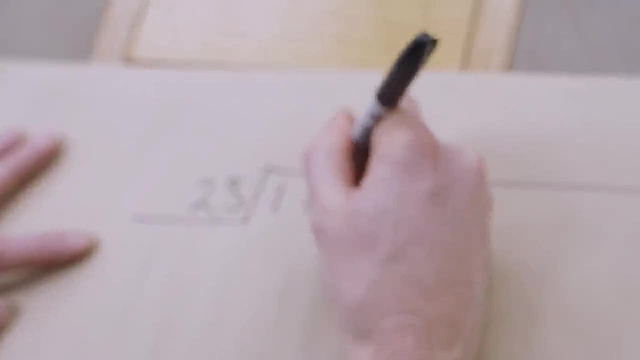 So in this case, straight out of the gates. one point: we're going to have to start putting some 0s on. It doesn't go into 1.. It doesn't go into 10.. It does go into 100.. 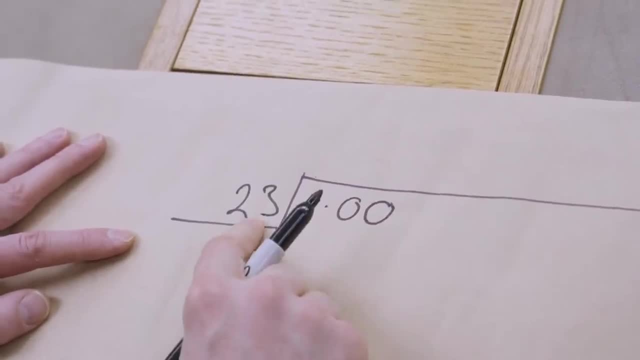 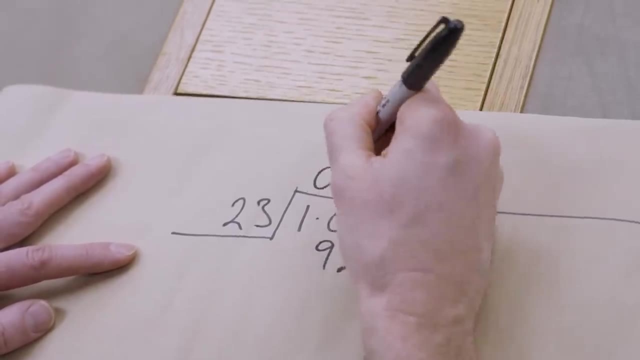 And you're like: well, how many times? Yeah, I think probably 4.. And you're like: and 4 times that is going to be 52. And then we did that 4 times. So this is actually our answer: 0.04.. 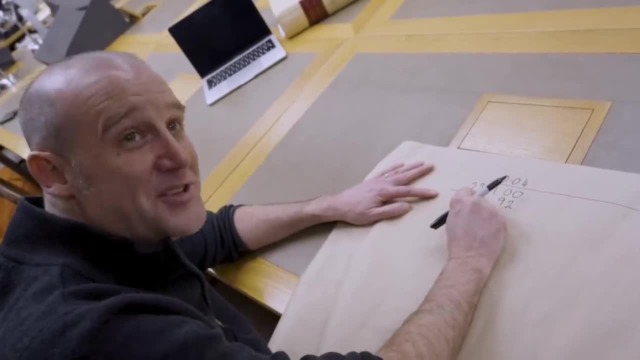 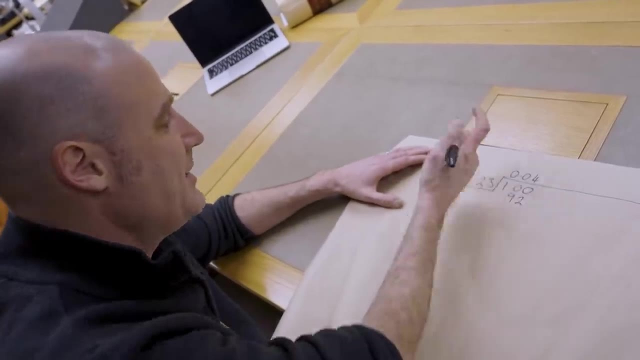 We're just trying to find a number in the 23 times table. that is the biggest, but not bigger than whatever our remainder is at the time. So what I'm actually going to do over here, I'm going to write out my 23 times table, if that's okay. 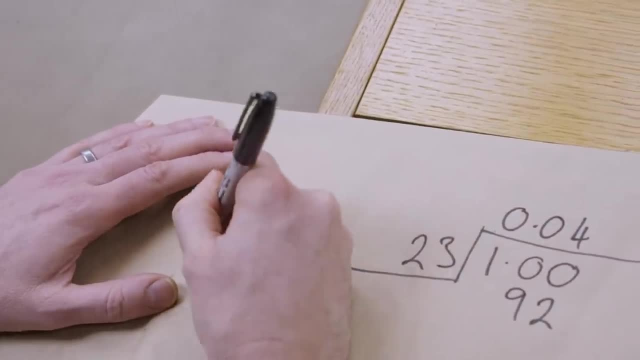 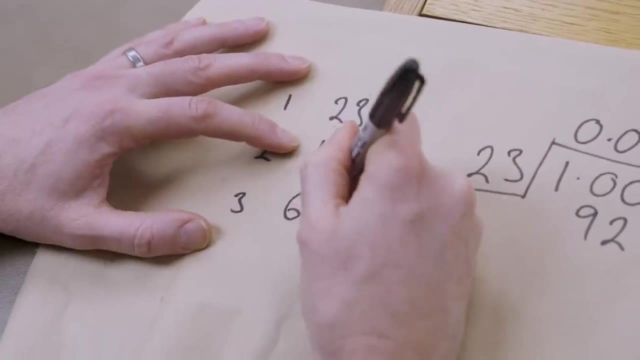 So 1 times 23 is 23.. 2 times 23 is 23.. 2 times 23 is we just double that 46.. 3 times 23 is add those together, which is 69.. 4 times 3 is just double what 2 times was. 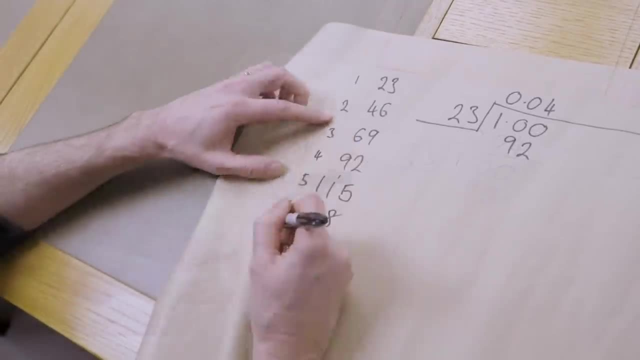 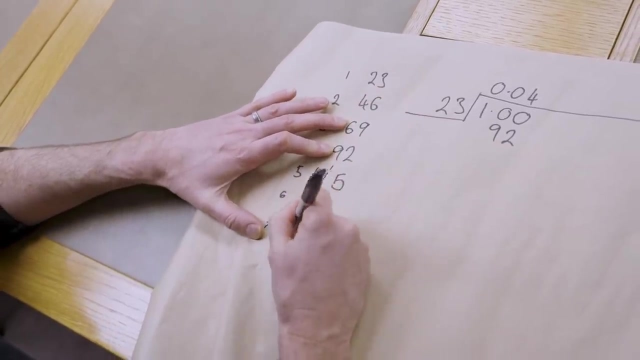 So that's 92, which is what 1- we've already used there 7 times- is. add 3 and 4 together, So 9 and 2 is 11.. 6 and 9 is 15.. 1 is 16.. 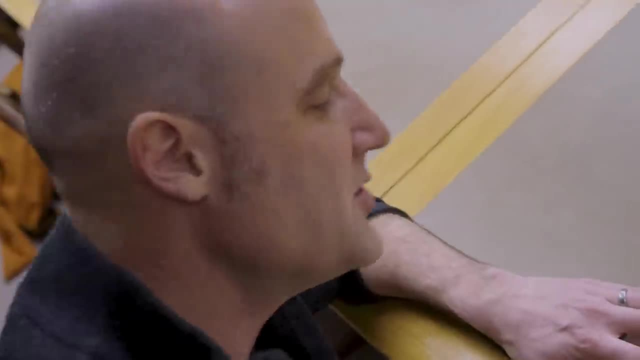 Wouldn't it just be easier to add 23 to that? Or you could just add 23 to the previous one. Okay, I'm going to be honest. Brady, You're absolutely right. Yeah, And what I'm actually doing is: 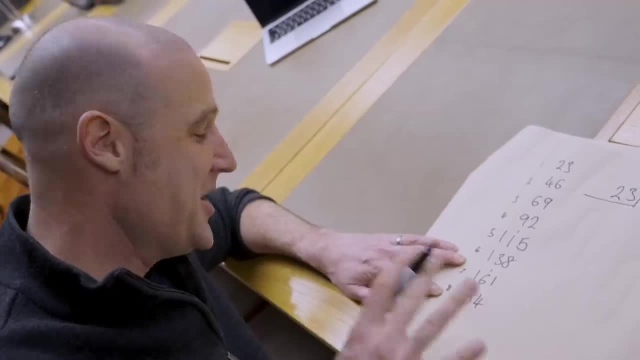 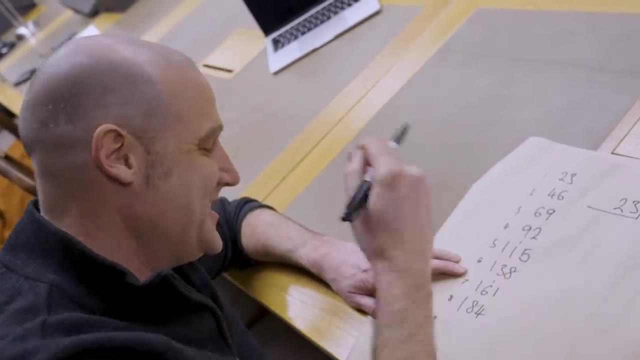 because I've done this on a much, much bigger scale. when calculating pi by hand, I was doing this for like 20-digit numbers, And so I've just gotten in this formula. You're right, I got so obsessed with my silly way of doing it. 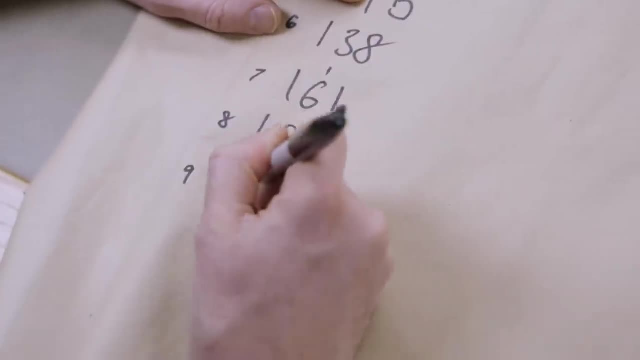 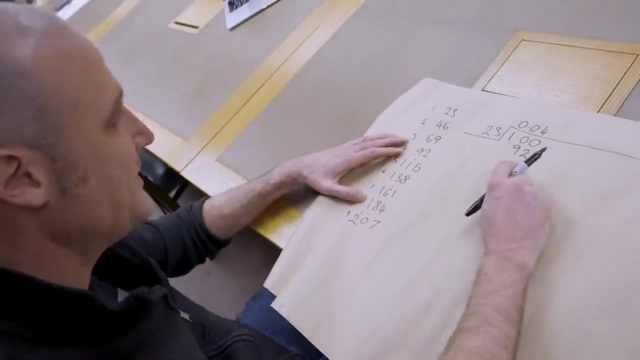 that I didn't stop and think: is there a better way? Okay, there, it is Cool. And if we add 23 again, we'd be up to 230.. So that's 10 times Okay. So this is going to speed up filling it in a lot. 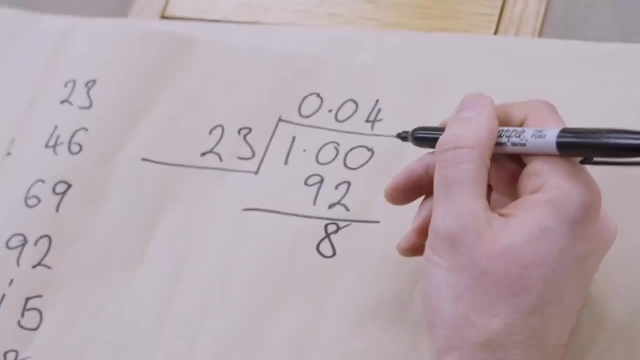 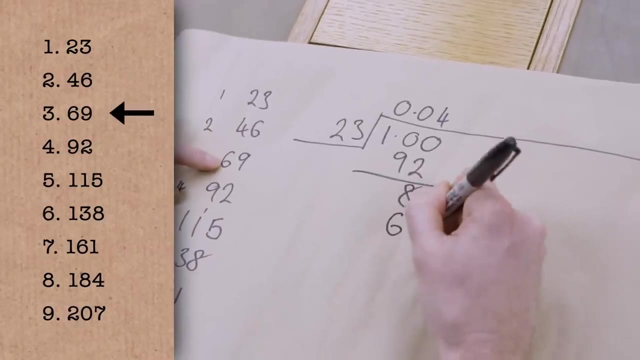 Then we subtract that off, That's 8.. Okay, so now it doesn't go into 8.. It does go into 80.. 69 is the biggest one we're going to have, And that's a 3. Subtract that off. 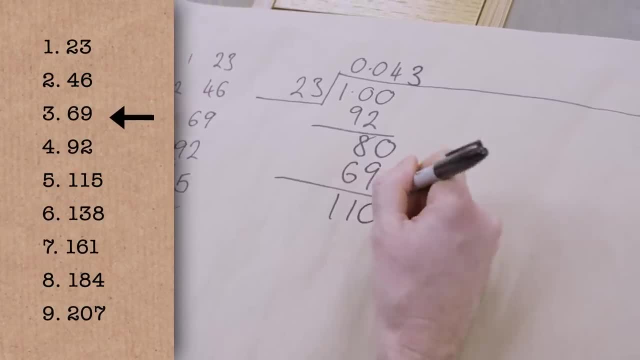 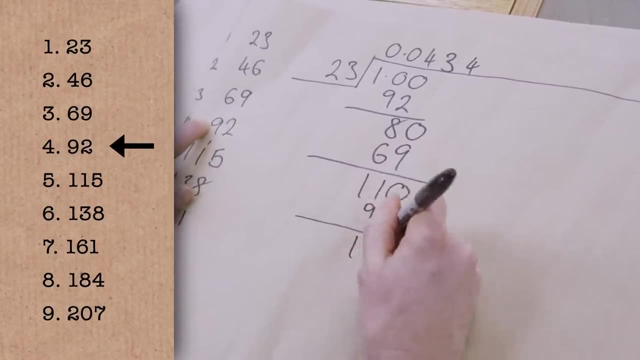 We're left with 11.. It doesn't go into 11.. 110.. Yeah, 92. And that's 4 times. Let me subtract this off, That's going to be 18.. It doesn't go into 18.. 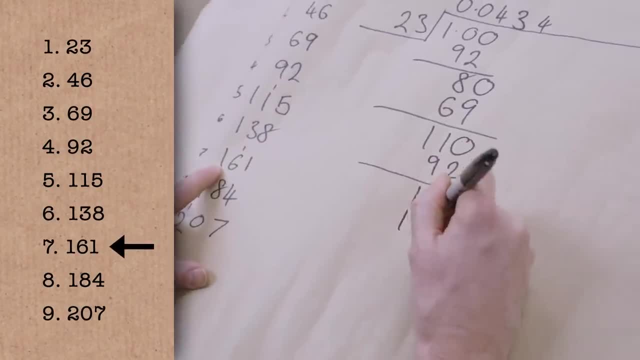 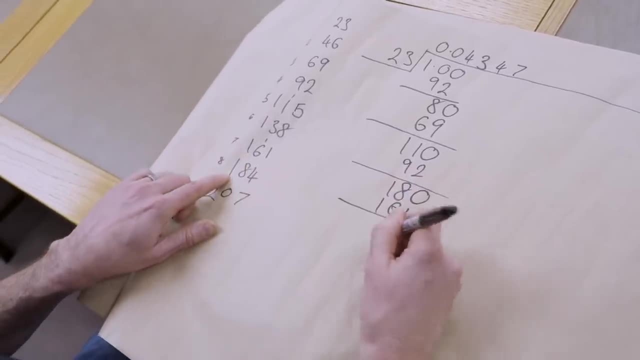 180.. Yes, That's going to be 161.. 161 is the next biggest one: 7 times, As you can see once you get into the swing of this: 19. 190.. 184.. 8 times. 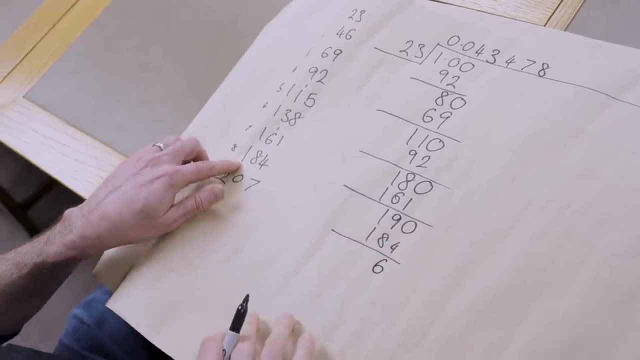 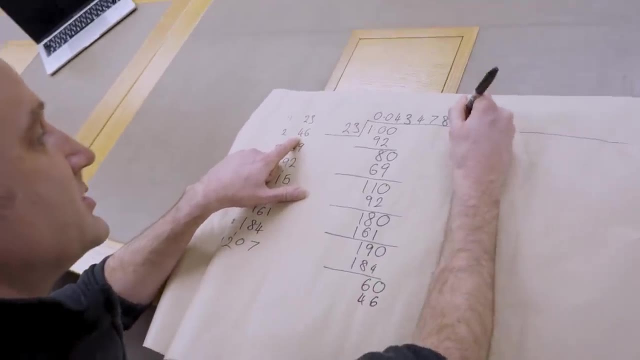 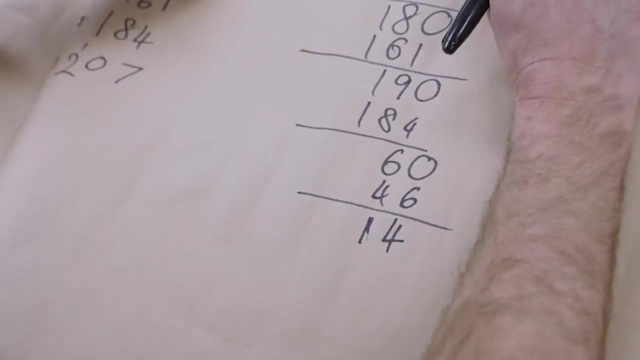 Subtract that off 6.. So now what we're looking for is, the first time, 60. Yeah, 46. Twice The first time we have a point where this remainder is one we've seen before. So we're at 14 now. 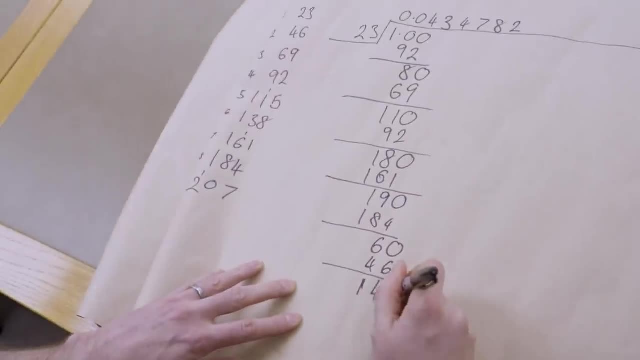 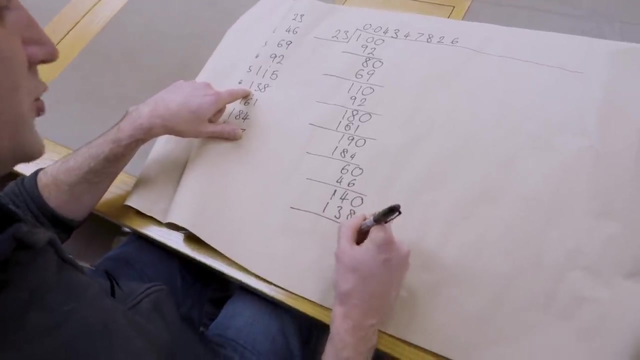 And we've never seen 14 before, So I've got to do 14.. And it's going to be 138.. That gives us a remainder of this time just 2.. So we've seen 2 before. We haven't. 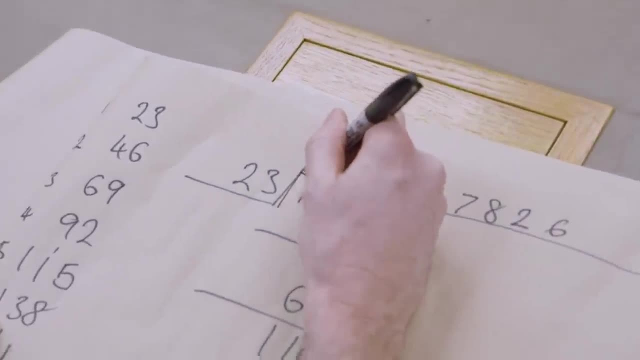 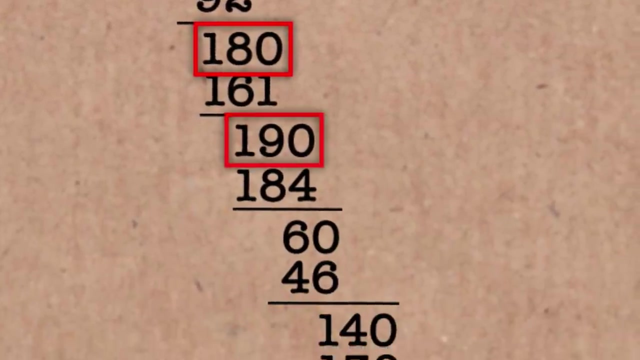 So the numbers we care about are the top ones, which are the remainders each time. So so far, we've seen 100.. We've had 80.. We've had 110.. We've had 180.. We've had 190.. 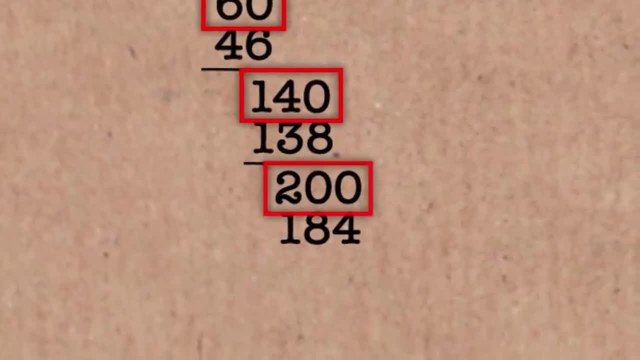 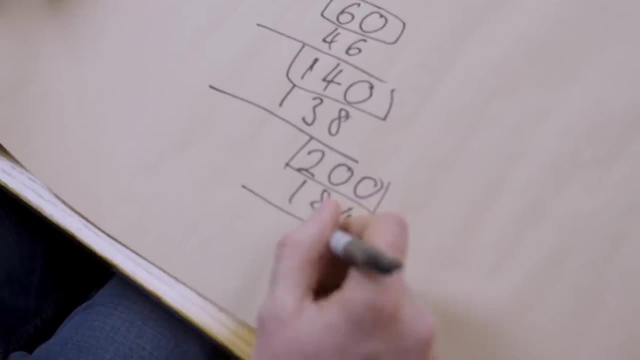 We've had 60. We've had 140. Now we've had 200. Then we said that 200 is 184, is 8 times Putting that up there, Remainder here is 16.. Have we seen 160 before? 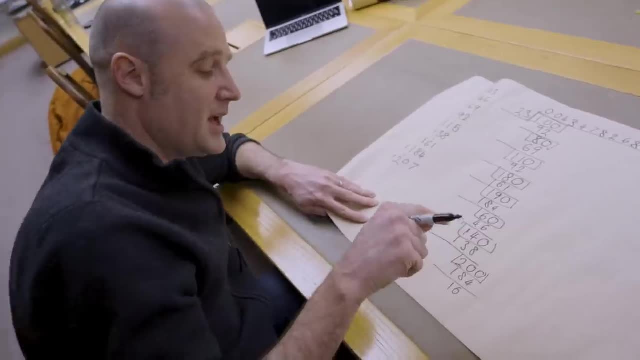 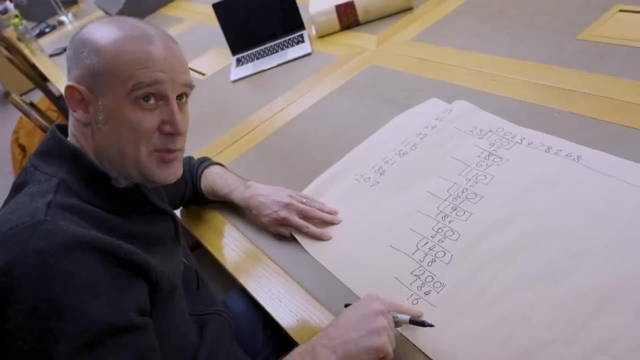 No, we haven't. So now we keep going. Now the question becomes: how long can we keep going? And each time we go we add one more here until we have to hit a repeat. Well, in this case ignoring the padding zeros, if we just take the non-zero bit, that's actually. 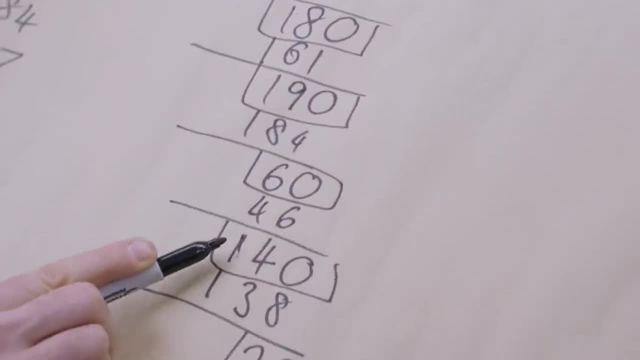 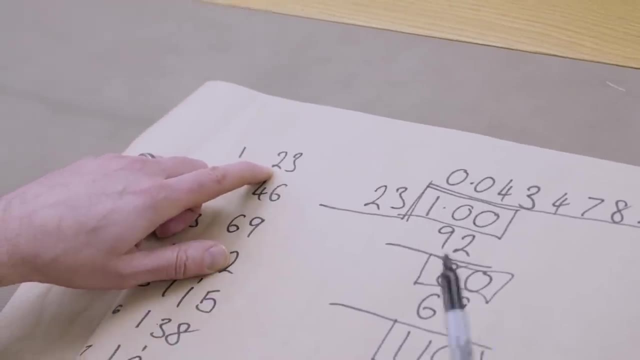 1,, 8,, 11,, 18.. 19,, 6,, 14,, 2. Those that can't be bigger than 23, because if it was bigger than 23,, we would have just picked a bigger number underneath and taken off one more lot of it. 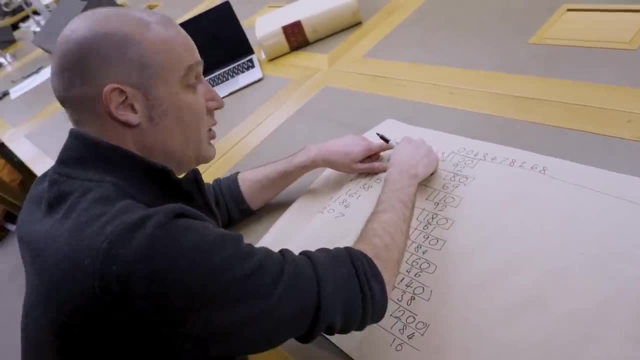 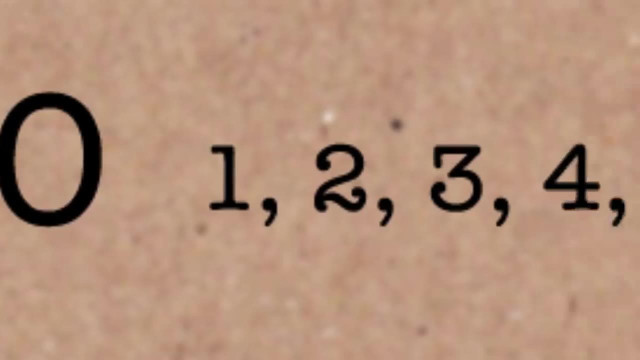 So the remainder, ignoring the zeros, is always smaller than 23.. So it can't be 0., It can't be 23. But it can be. any of the numbers in between, all the way up to 22, can appear in here. 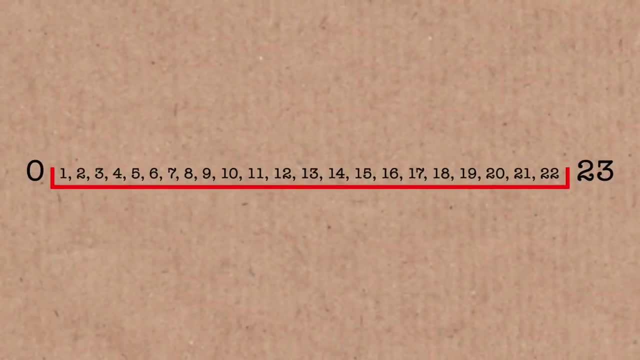 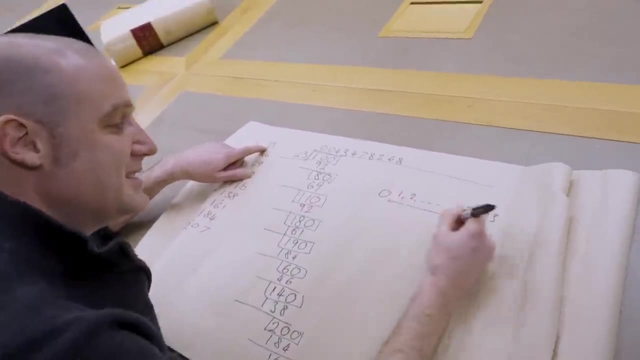 That's fine. It can be. any of the numbers in between, all the way up to 22, can appear in here. That may not all appear in there. We may hit a loop point before we get there, Or they may all appear in there somewhere. 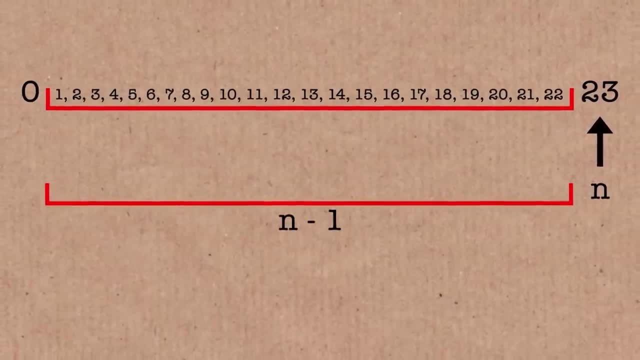 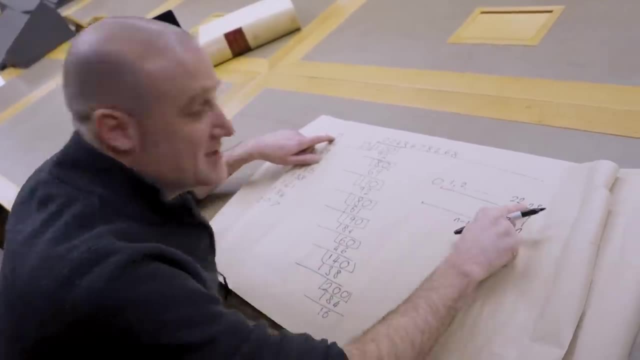 And if we just redid this as n, then the number of options before it is n minus 1.. And so that's your worst case scenario: is it's going to take n minus 1 steps. Once we've done that, we've used every single one. 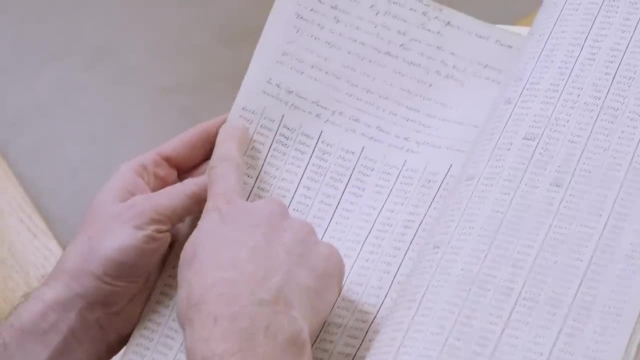 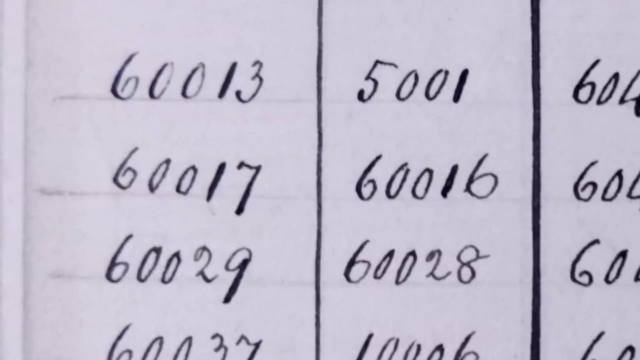 The next one has to be one we've used before We'll hit a loop point. We see here 60,017.. That was as bad as it gets. That was 60,016 digits, So it hit every single one of them before it finally repeated. 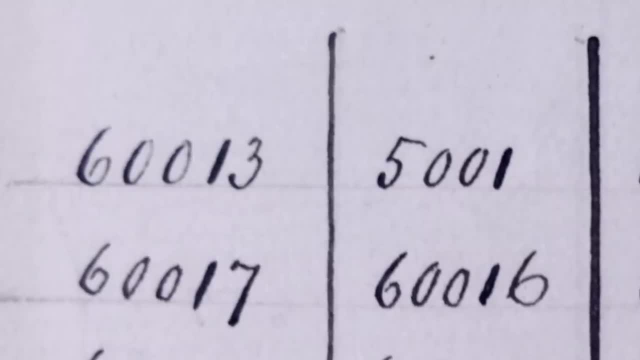 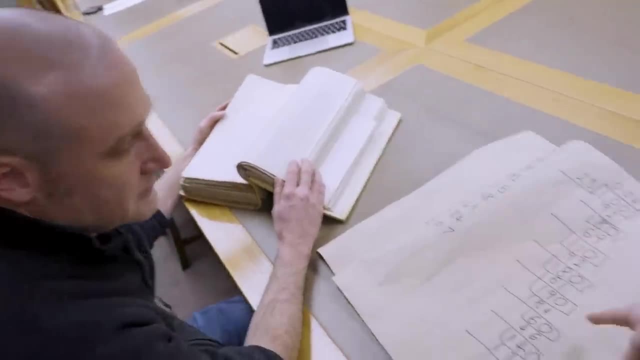 Whereas the one before it only hit 5,000.. It hit less than 10% of the possible values before it hit a loop point. Surely Shanks wasn't doing this for all those messages. You know what? I don't think he was. 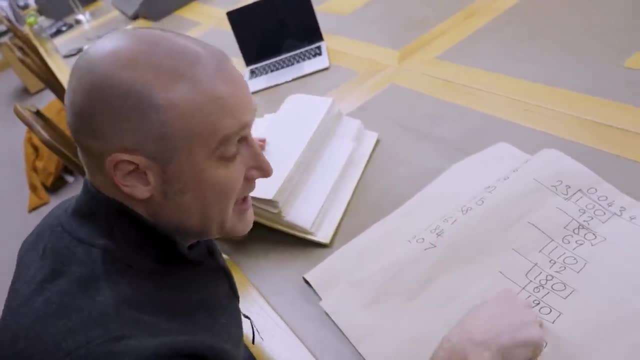 Because, Partly because, Partly because this takes a really long time, And you can see me doing it- The first thing you've got to do is you've got to generate your table, And then you've got to go through and do this. 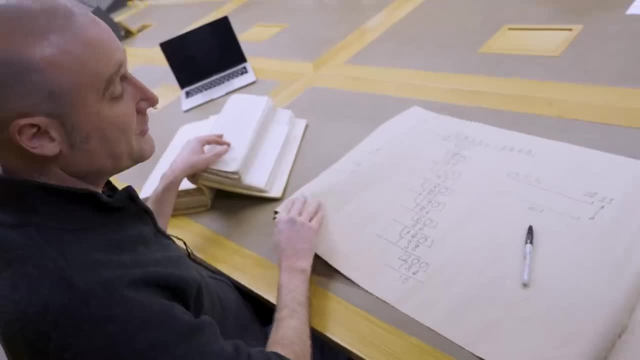 And, as you can see the way I'm doing, it takes up a lot of paper And for a small number And for a small number And what you can do when you get here. So I've done a little long division of my time. 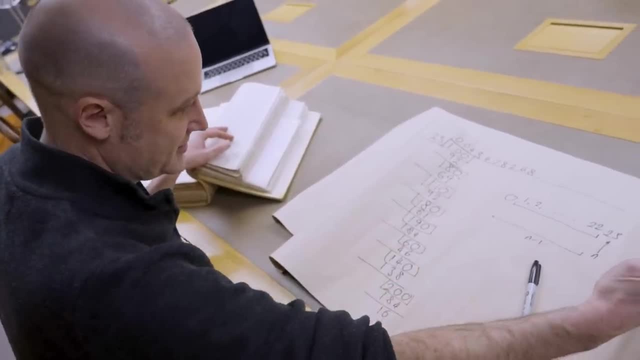 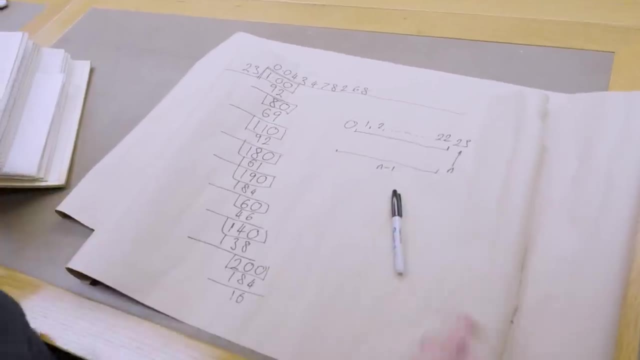 What we did was: you want printed paper with squares on it, so everything stays lined up, And then, when you get here, you copy it up and then you do another stripe, And then you copy it up and you do another stripe. But you're still going a long way that way. 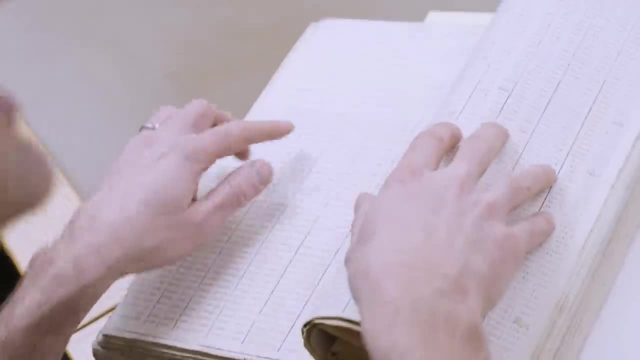 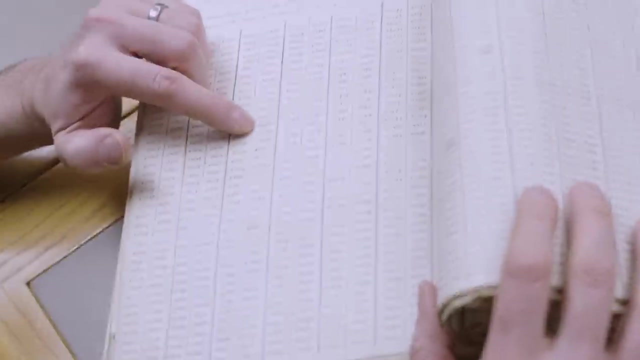 And you can't imagine. he went 60,016 digits in that direction. That's one clue. he didn't do it this way. The other clue is the type of mistakes he made Here. he thought it repeated every 30,525.. 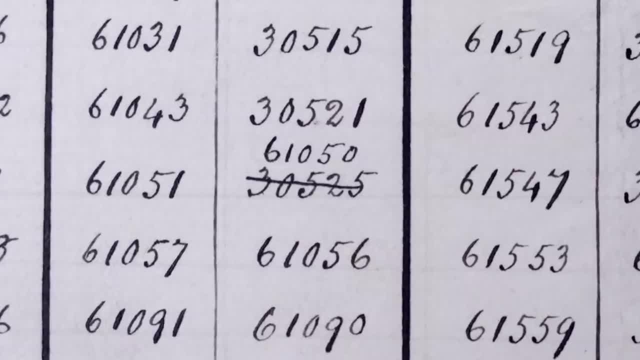 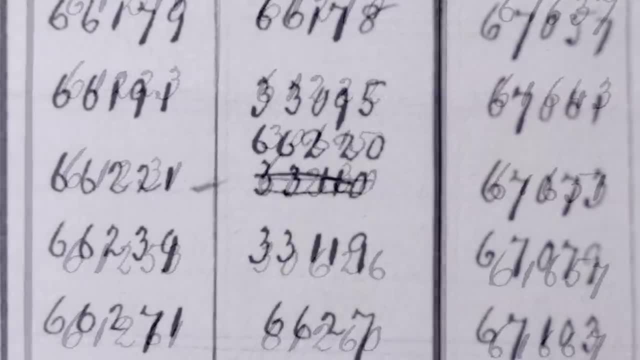 And he corrected it to 61,050, which is exactly twice what he thought he had. If you look at all these corrections, he's always either doubling or halving it, Which makes me think he's got a technique that probably involves powers of two or something. 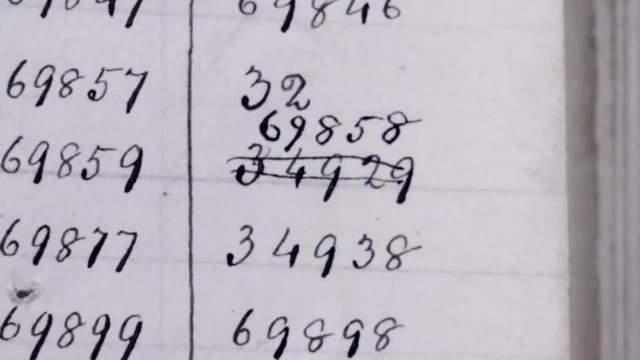 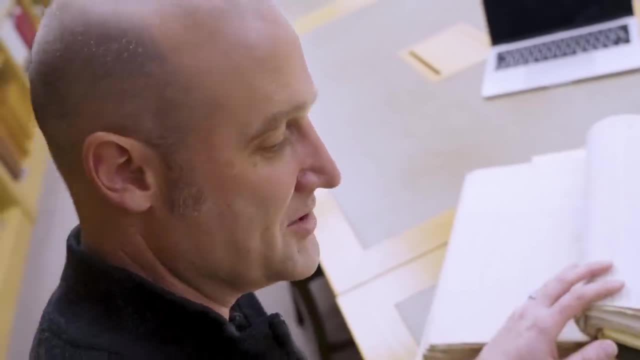 Or something Or some steps of halving, And sometimes he's done one too many or one too few, And that's what he's corrected. So that kind of systematic error leads me to believe he wasn't doing it this way. He had another way of doing it. 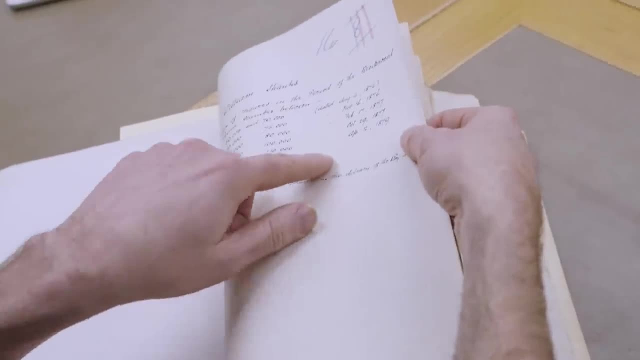 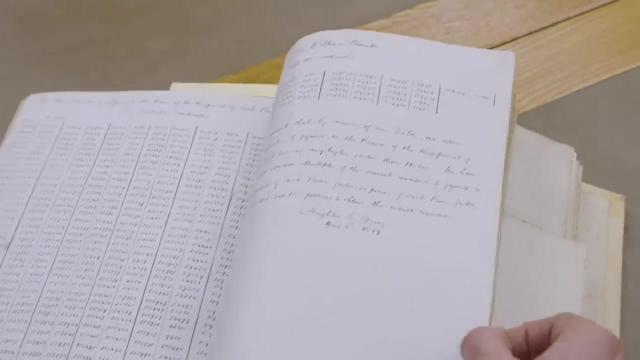 He died in 1882. So this is like three years before he died. He's still sending in, He's up to primes, up to 110,000.. So where did he get to on this one? Oh, there's a note at the end. 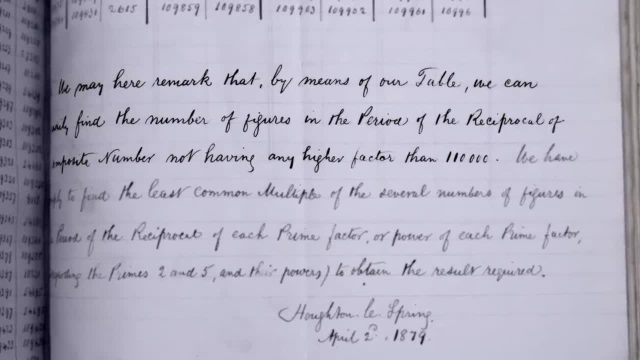 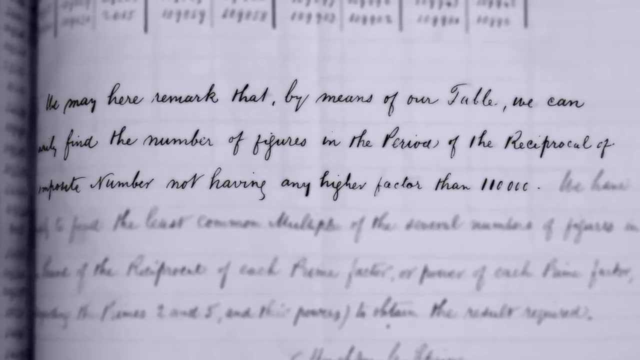 Note. We may here remark that by means of our table we can readily find the number of figures in the period of the reciprocals of a composite number not having any higher factors than 110,000.. So he's basically said these are useful because you can use the reciprocals of the primes. 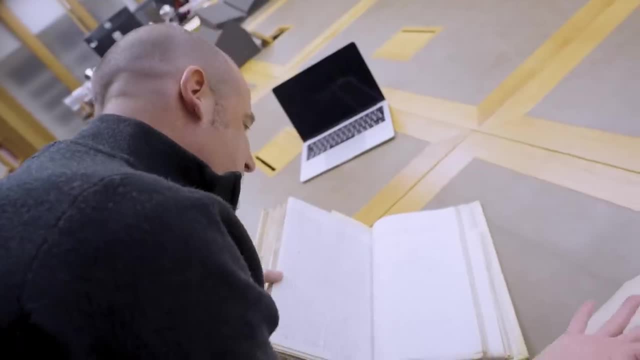 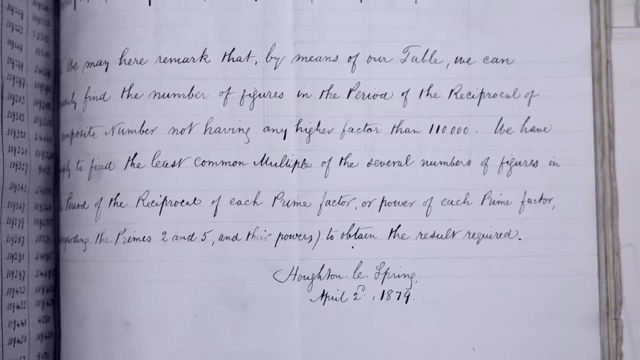 to get all the reciprocals of the composites, Doesn't say why that's useful. We have simply defined the least common multiple of several numbers of figures, And he explains how to do that, And then he signs off His only practical application for what he's done. 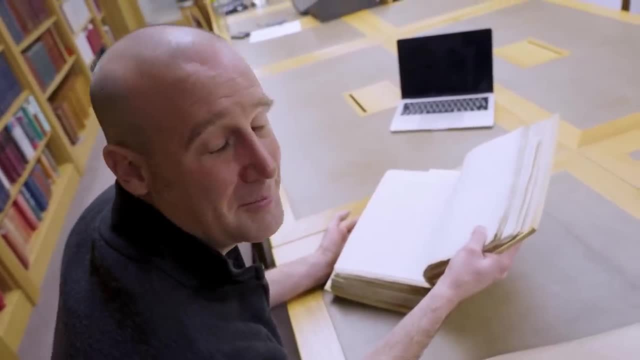 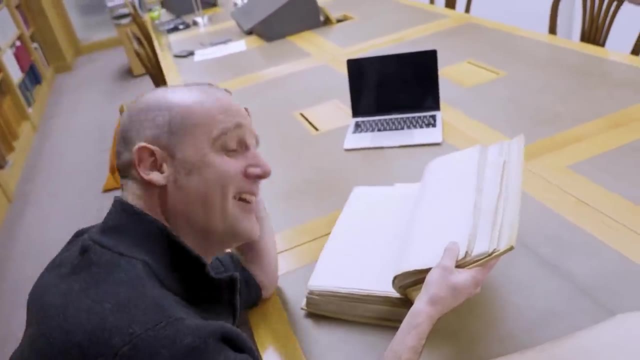 is, you can use it to find another thing with no practical application. Nice, I like this guy. Yeah, I like the cut of his jib. Imagine how good his YouTube channel would have been. He definitely would have had a YouTube channel. 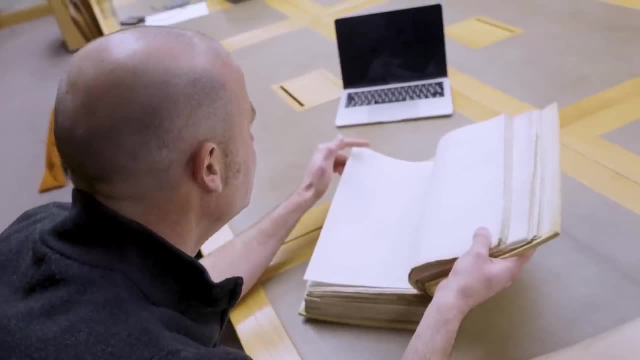 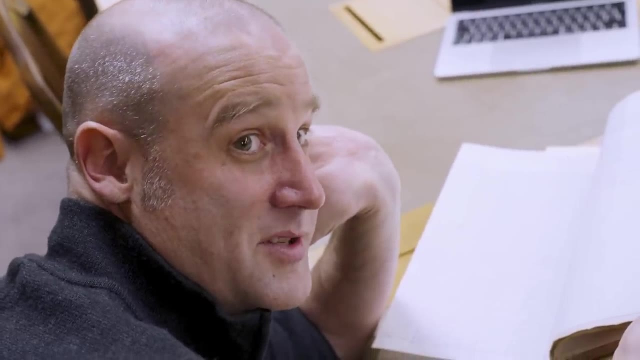 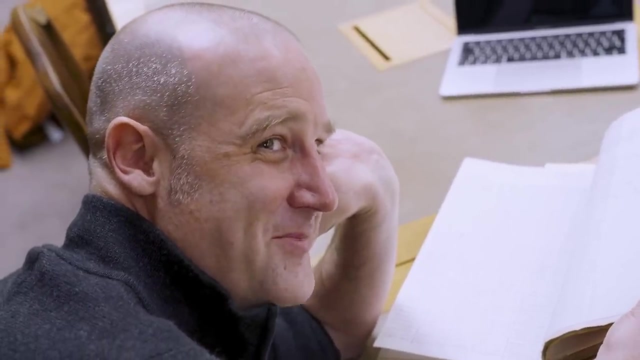 Yeah, What would he have thought of the shank bot? Well, I don't know, Because if his sole goal was to find these numbers, he would love shank bot. I feel like it was the doing that he enjoyed, And I feel like the fact that I coded it up. 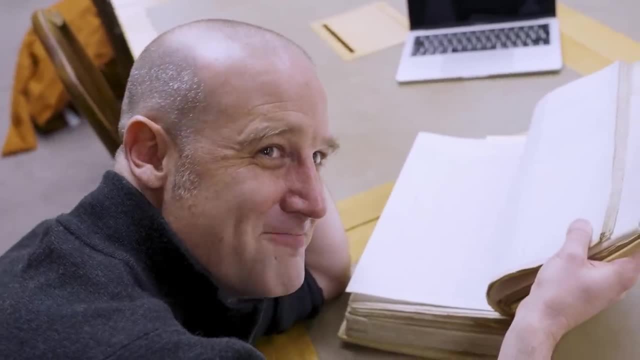 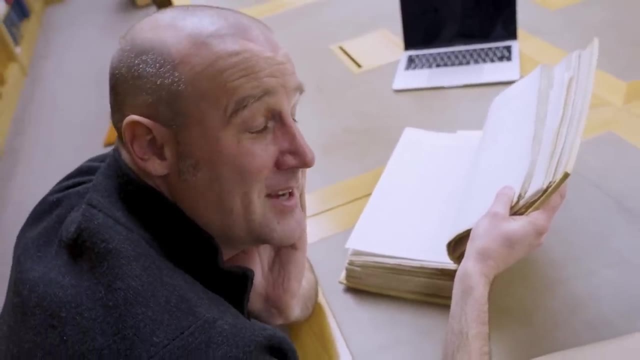 and shank bot just kicks it out without flinching, Not the same One. last question, because I know you've been doing a lot of research into him: Was he married? Yeah, Yeah, And his wife survived him by a good 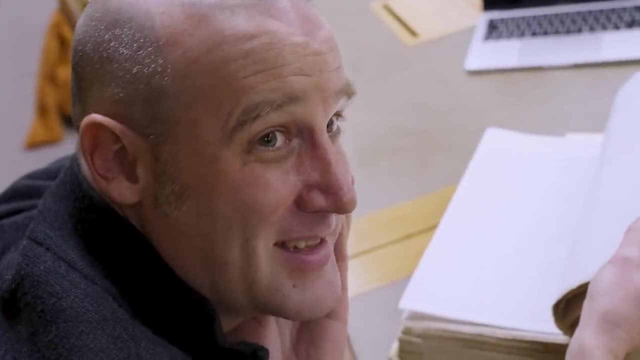 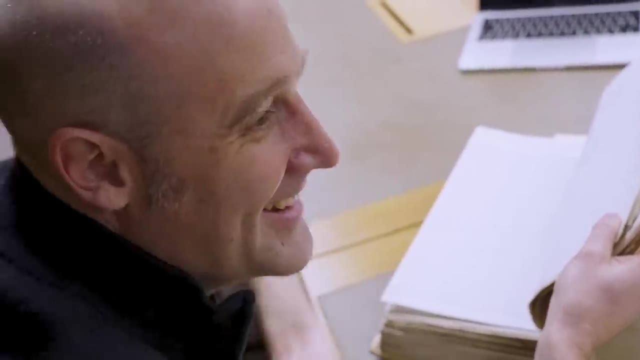 pretty much two decades, Yeah. So he was like every morning he's like morning honey, I'm off to work. And by work he would just walk upstairs, start doing calculations, Like, oh, another hard day in the office. 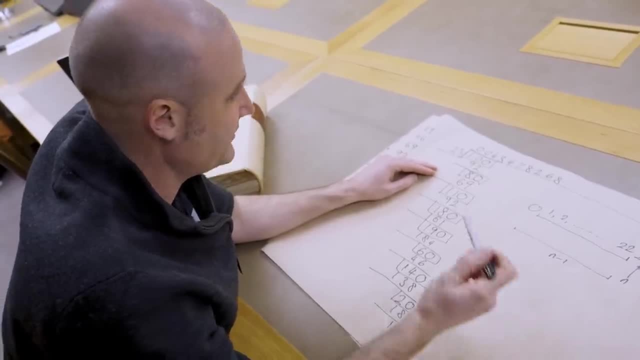 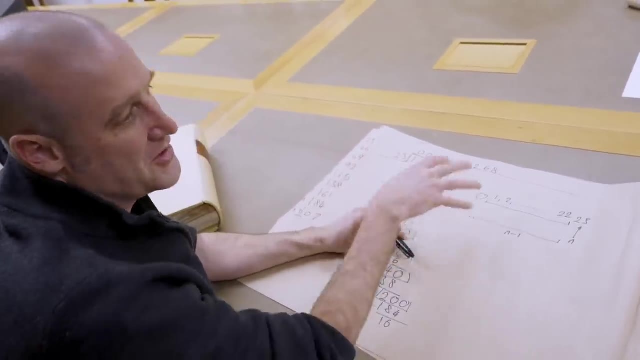 There are some obvious follow on questions that you can have at this point. You could ask yourself: do you take the reciprocals, or at least the length of the repeating part of the reciprocals of the primes, and use it to work out? 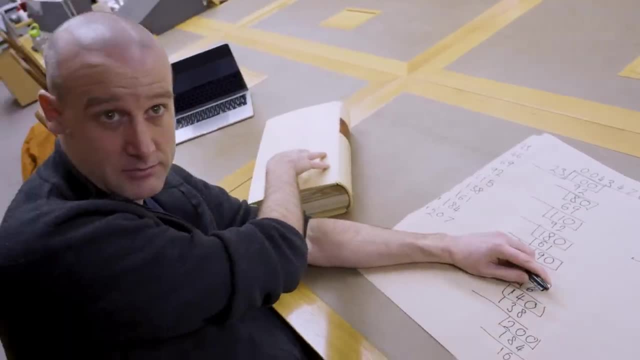 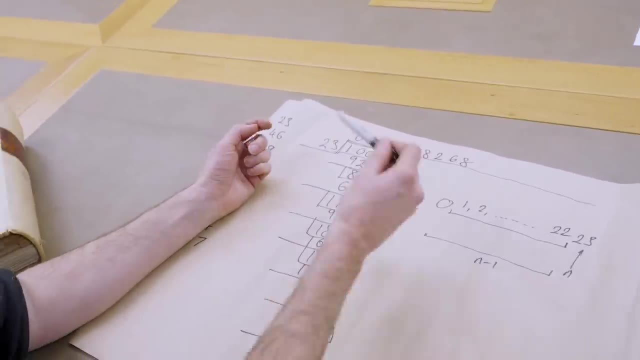 the repeating part of the reciprocals of composites, which is what shank's put in there as a little note. You can also ask yourself what's special about the numbers like seven that use every single one of these before they get back to where they started. 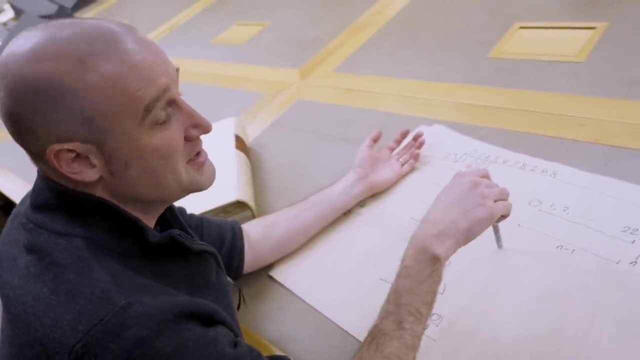 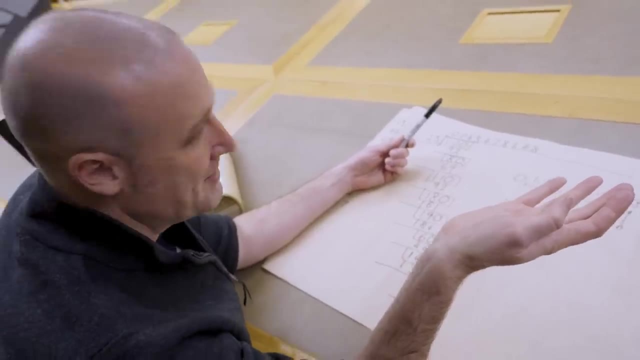 And it turns out it's something called you've got a thing called a primitive root, So prime numbers don't have factors, but they can have primitive roots, which involves doing powers of things and remainders And primes that have 10 as a primitive root. 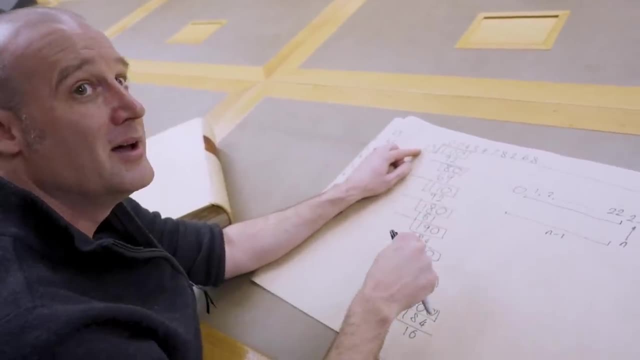 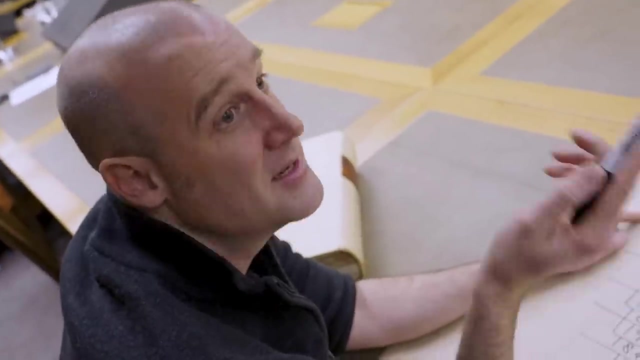 will have every single one of these pop up Because 10 is their primitive root. they go through every single one before they get back to the first one, which is why 60,013 does not have 10 as a primitive root, So it only used 5,001. 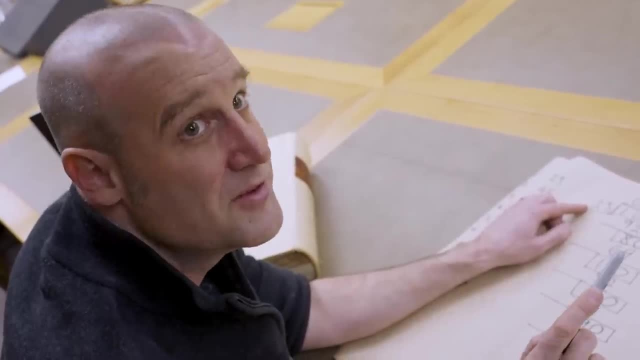 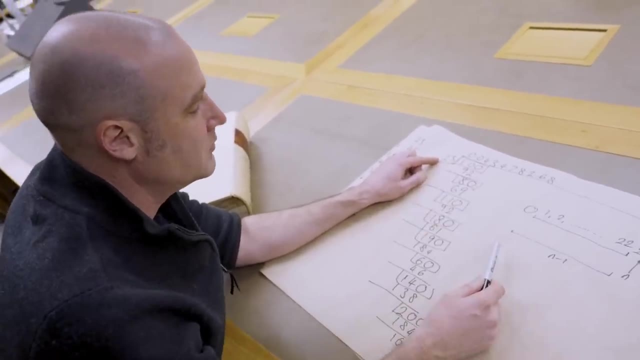 And then 60,017 does have 10 as a primitive root And that's why it took that long. It used every single one before it got back to where it started. And there's a thing called the Reptend prime which also tells you. 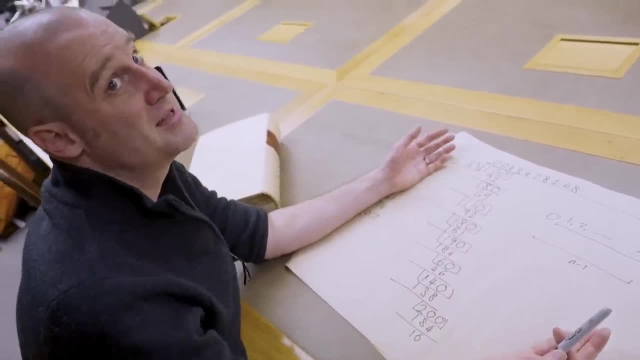 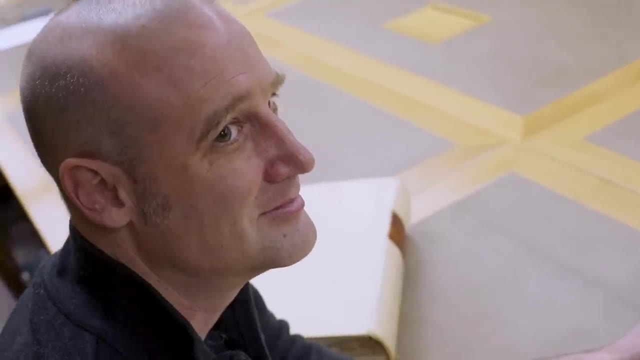 the ones that have this incredible property, So if people want to look into it, there's a lot more fun For me. however, all about the long division, So just so I'm clear: 60,017 and 7 are Reptend primes. 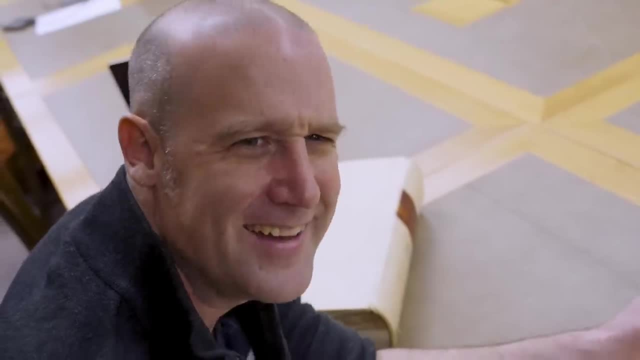 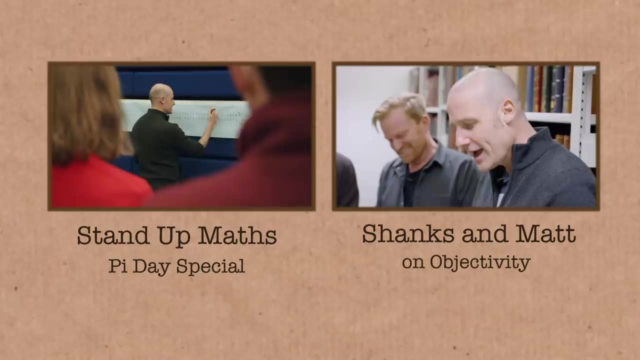 Yes, Because they go to the max. Yeah, yeah, yeah, I will allow that as a definition. Right, Right, If you like this video, you're really going to like Matt Parker's new video on Pi Day 2022.. 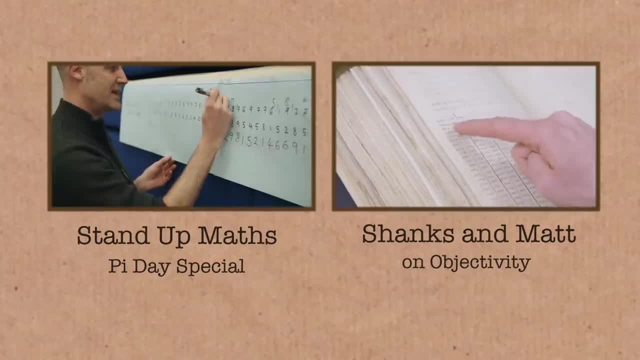 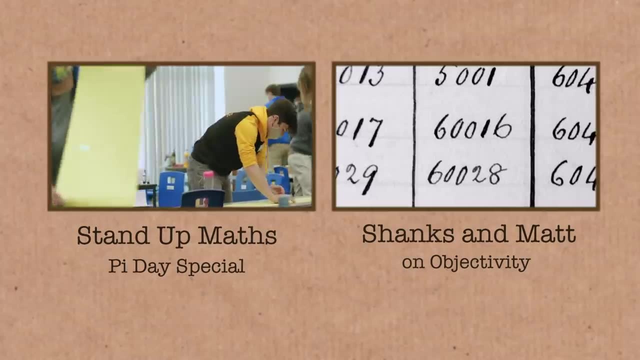 It's on his channel, Stand Up Maths And also Matt, myself and Keith Moore from the Royal Society talk more shanks on the Objectivity channel. There are links here on the screen and down in the video description: Hero- Yeah. 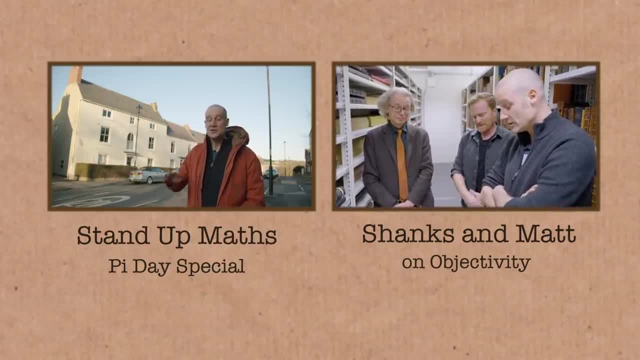 Hero, Northumbrian hero, Yeah, And still world record holder for most digits of pi calculated by hand.